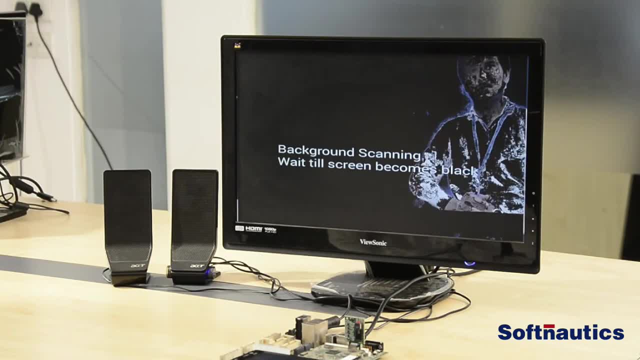 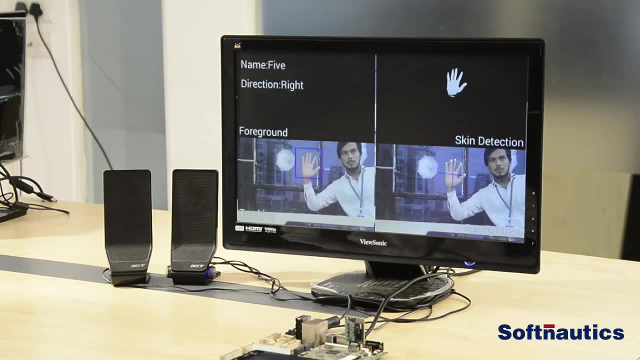 of an Android application. As you can see, it is currently performing background scanning till the display becomes black. Then it goes for hand-scanning tuning, where user map his hands with the shown image to adjust to parameters. Now it has started to detect and track gesture with 5 fingers. 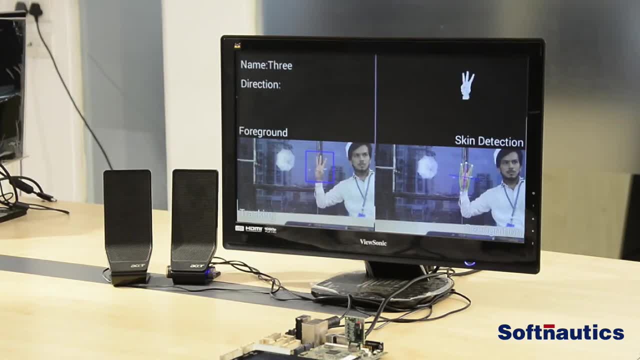 and appropriate gesture name is displayed. Let's change the gesture having 4 finger, gesture having 3 finger, gesture having 2 finger and accordingly the appropriate names are displayed: 5 fingers down, 5 fingers up, 3 fingers left, 3 fingers right- and appropriate action is. 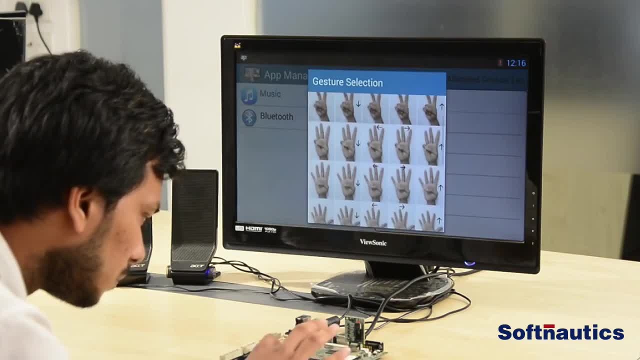 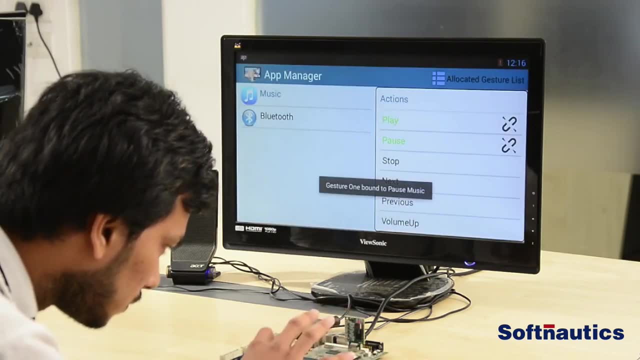 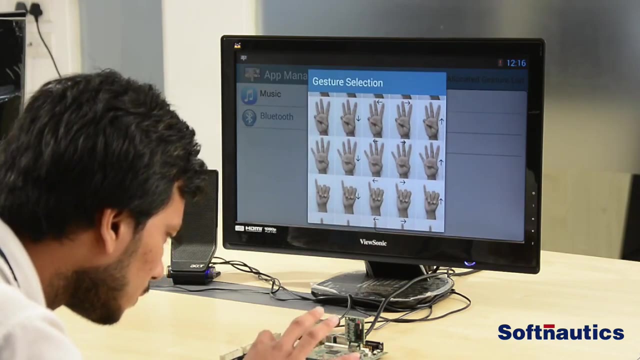 displayed. Let's see the binding of hand gesture in AppManager. To bind play event, click on play. it will pop up gesture selection list. Select on any gesture from the list. Click on pause and select appropriate gesture. Click on Bluetooth and select appropriate gesture for on and. 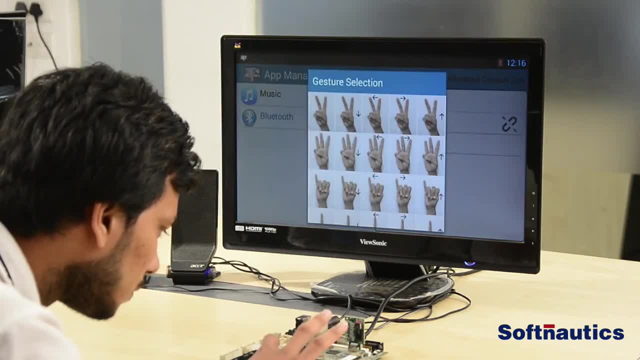 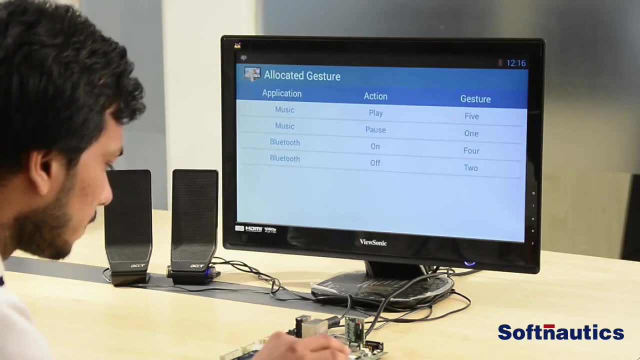 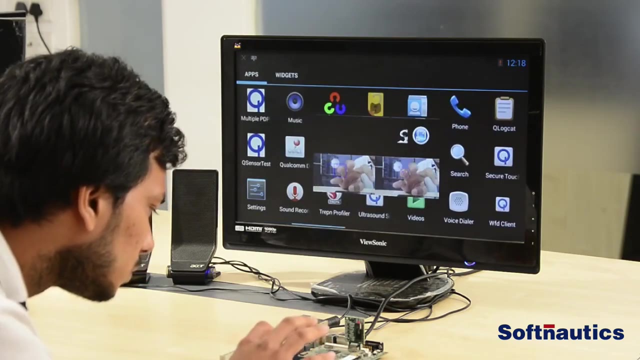 off event respectively. Click on allocated gesture list to see the gesture mapped with application events. Let's start the application in floating mode. Floating mode allows you to reposition the app anywhere on the screen. Let's start the music player application and perform play pause using hand. 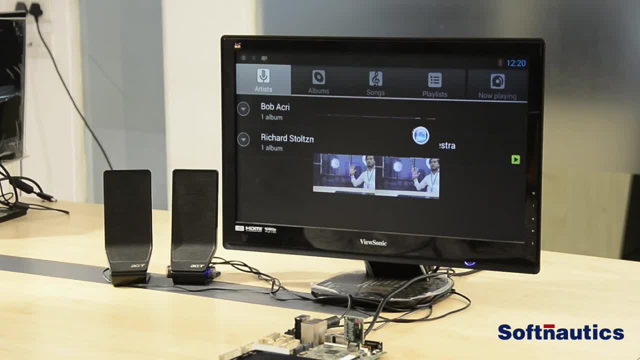 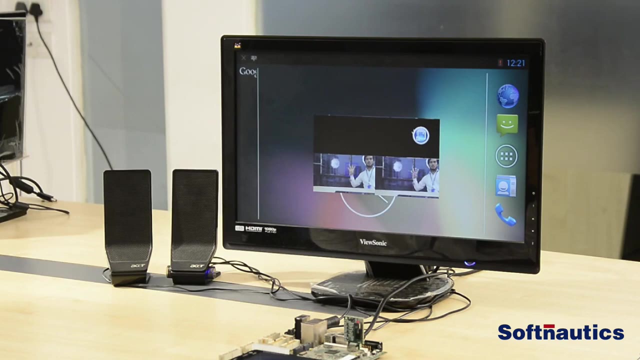 gesture, Let's go back to the home screen. Similarly, let's control the Bluetooth on off events using hand gesture. Hand gesture recognition library runs at 30 fps on ARM and Hexagon Q ESP core of Snapdragon platform with 640 x 480 frame resolution By splitting algorithms. 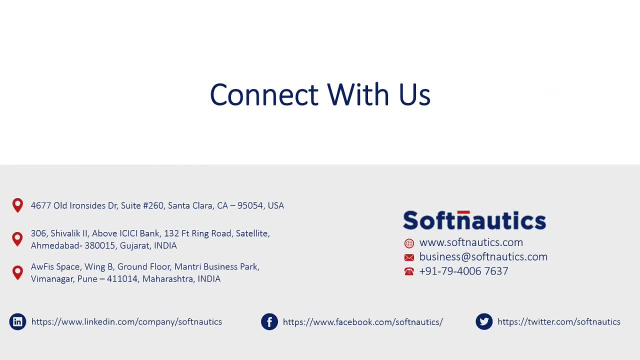 between ARM and ESP, core power saving is achieved, since ESP runs at much lower frequency. Thank you. Subtitles by the Amaraorg community.